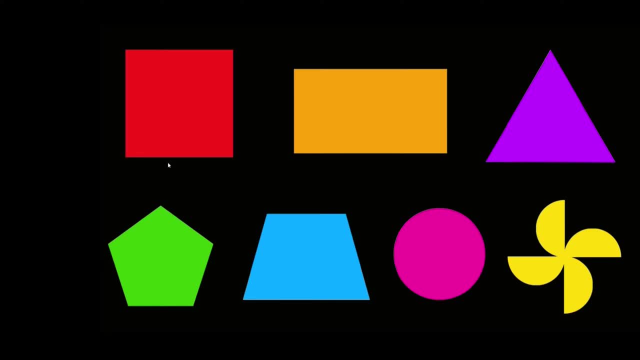 them are the exact same angle, right? These are all 90 degree angles, okay? And a quick way that you can figure out what the angle of rotation is for a shape. well, remember, a full rotation is 360 degrees, right? So let's just start there. A full rotation is 360 degrees, okay? So if you 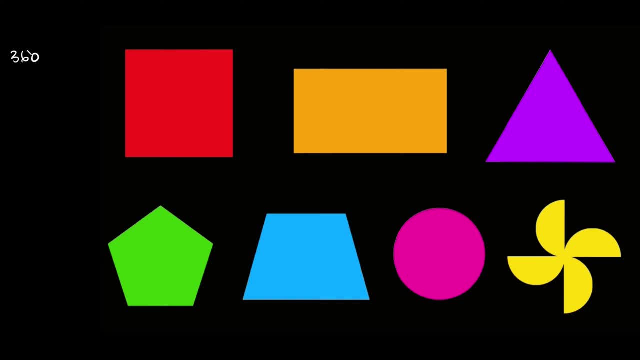 want to figure out, for example, this square, all you'd have to do is 360 divided by however many corners you have on your shape, right. So the square has four corners right, or four angles, or four vertices. So we're just going to do 360 divided by four, okay, And that is equal to 90. 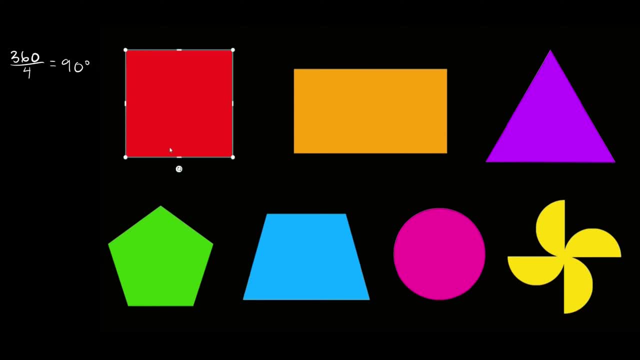 degrees, all right. So again, that means, if we rotate this thing 90 degrees, or every 90 degrees that we rotate it, it's going to map onto itself, right? So if we rotate it 90, it maps onto itself. 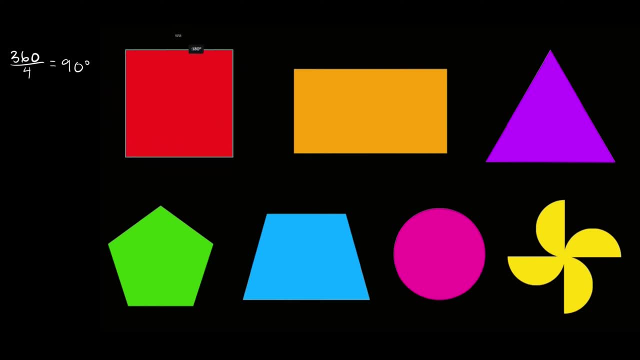 Oops, there's 90.. Another 90, right, Right there, And another 90. Right there, And then, lastly, this 90 degrees back to zero. Okay, so that's an easy way you can figure out the angle of rotation for a regular polygon. Now for something like this this: 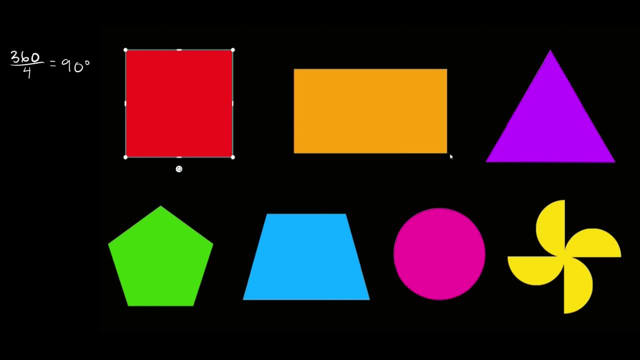 rectangle. this is not a regular polygon, right? Because all the sides right here are not the same length. So when we rotate it, you're going to notice if I rotate this thing 90 degrees, it's not going to map onto itself at all, right? So what we have to do is rotate it another 90 degrees. 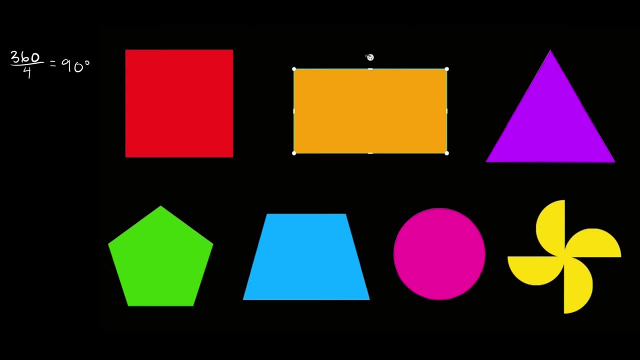 right. So this rectangle does have rotational symmetry, right, Because we were able to map it back onto itself by a rotation of 180 degrees or less. okay, So the angle of rotation for this rectangle would be 180 degrees. all right. Now here we have an equilateral triangle, right? So 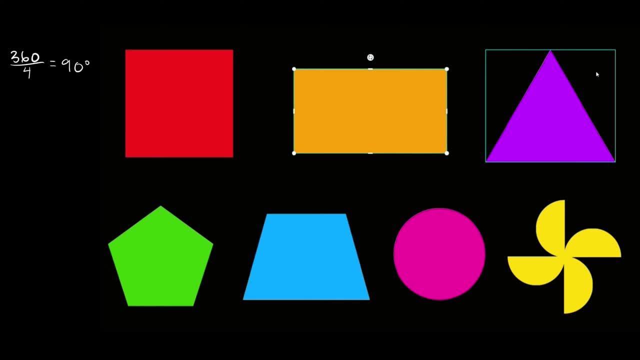 that just means all the sides and angles are the exact same, which also means it's a regular polygon right. So if we want to figure out the angle of rotation for this triangle right here again, just start with the angle of rotation. So if we want to figure out the angle of rotation for this, 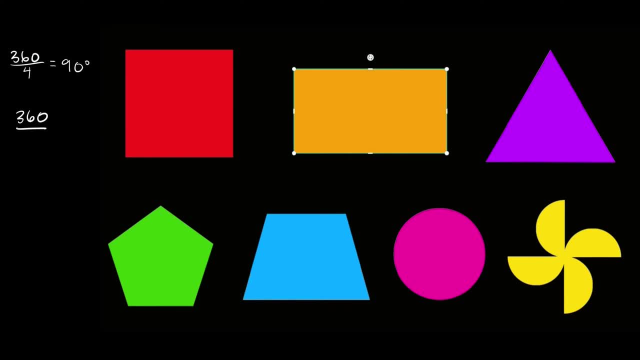 rectangle. we're going to start with 360 degrees and divide it by however many angles you have. So we have three, right? So 360 divided by three is equal to 120 degrees, all right. So that means, whenever I rotate this thing, 120 degrees, it should map back onto itself. okay, And you're. 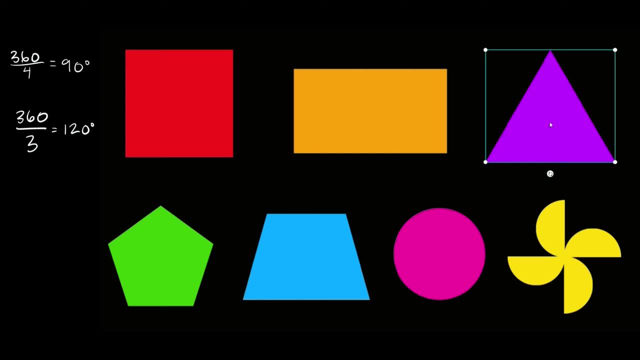 going to notice that it's actually going to come off a little bit because I'm not rotating it from the very center like I should be. I'm rotating it from the side, but it's going to be kind of the same thing. So again, if I rotate this thing 120 degrees, where's 120, right? 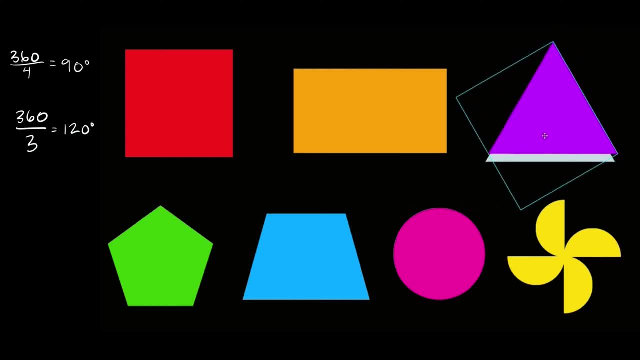 There. okay, As you can see again, it came off a little bit because I'm not rotating it from the center, but if I move it back to right there you can see it matches up exactly to where it started, right. And then again, if I rotate it 120 degrees right, Another 120 degrees, or a total of 240,. 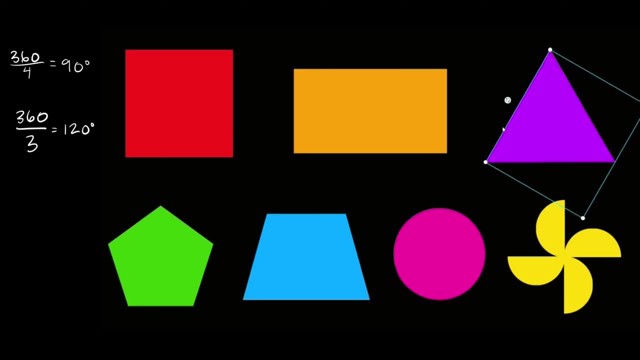 120. right there Again, you can see it matches up with where it started. okay, So this equilateral triangle also has rotational symmetry. All right, now let's come down here. So this one is a pentagon right Five sides. So, as you can see, it's a regular polygon right All the sides. 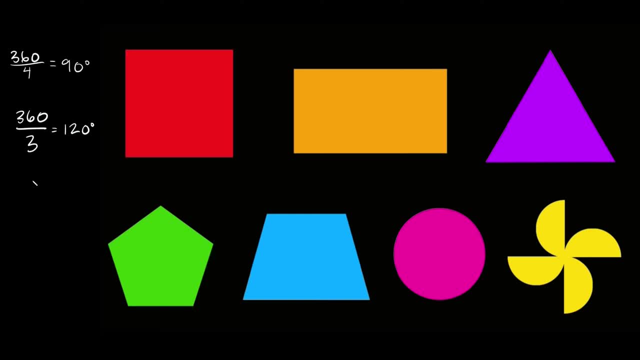 are the exact same length, and so are the angles, right? So if I want to figure out the rotational symmetry for this one, I'd do: 360 divided by 5, and that's equal to 72 degrees, right? So whenever we rotate this thing 72 degrees, it should map back onto itself, right? So rotate it 72 degrees. 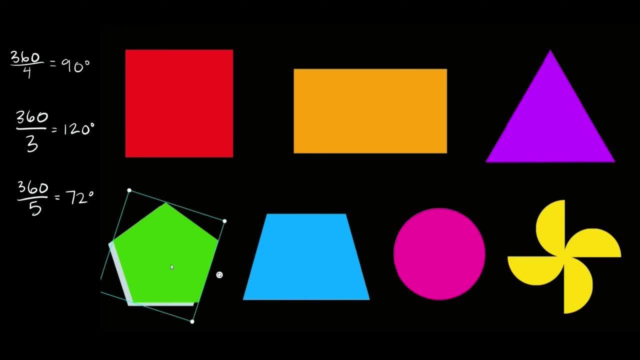 right there. but again, I'm not rotating it from the center. I'm off to the side a little bit, that's why it's coming off a little bit, but you can see it still matches back up to where it started, right. And then again, if I rotate it, another 72 degrees, so 144 degrees, 144 right. 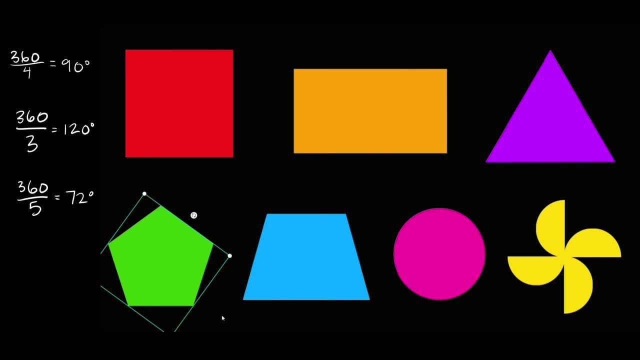 there and we'll scoot it back right there. okay, It matches up to where we started, And then we could do that going all the way around until we get back to zero. right here, right, All, right, now let's go to this trapezoid. So let's rotate this thing and see if it maps. 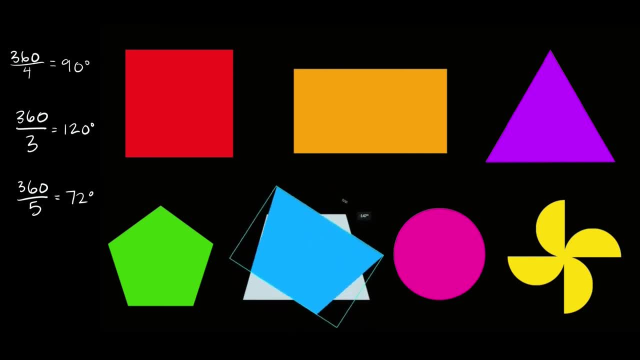 onto itself. No, no, no, no, no, no, no, still no. What about at 180 degrees? No, okay, So we rotated this trapezoid 180 degrees and it did not map back onto itself a single time, right, So that?